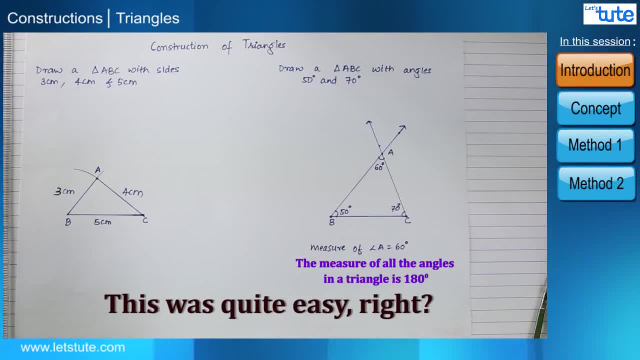 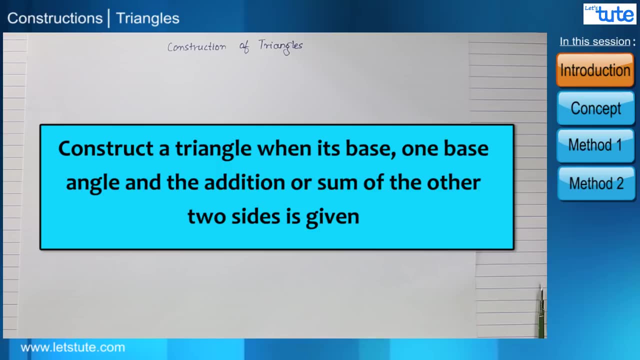 This was quite easy. right Now let's see a little complicated situation. Construct a triangle when its base 1, base angle and the addition or sum of the other two sides given. Now to understand better, let us take some numbers. construct a triangle with base QR as 5. 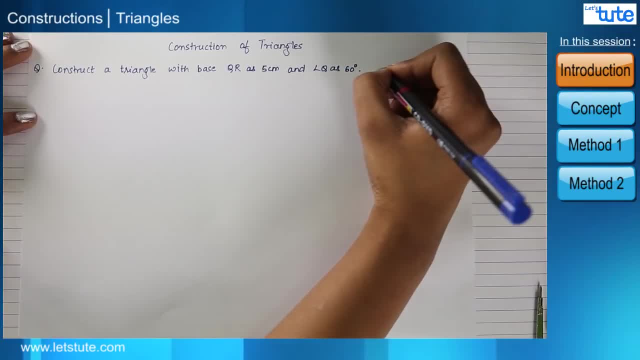 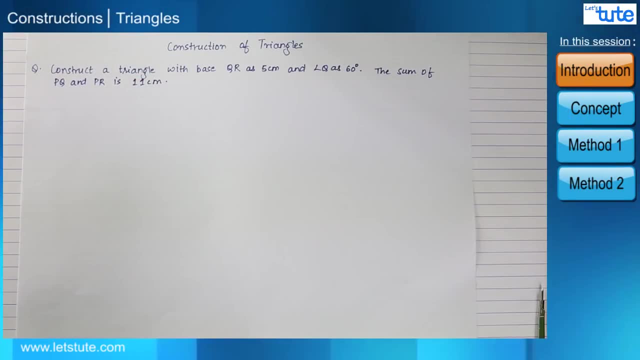 centimeter and angle Q as 60 degree, the sum of PQ and PR is 11 centimeter. let's first understand the logic behind this construction and how we are going to make it so. first, we are going to draw a base QR as 5 centimeter and make angle. 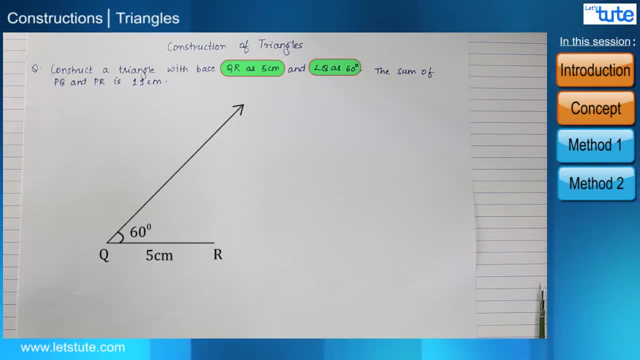 Q is equal to 60 degrees. now we are going to mark point a such that Q a will be equal to PQ plus PR. now what we have to do is to find or locate point P on Q a here. now we know that Q P plus P a will be equal to PQ plus PR. hence we can. 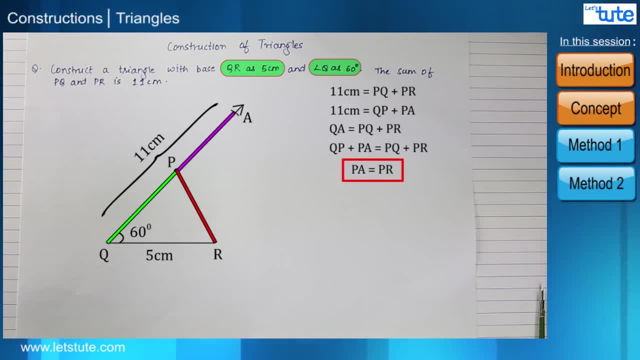 say that P a will also be equal to P R. now what ways can you think of to make P a equal to P R? well, if we will join a R and draw a perpendicular bisector of the same, then we can see that this perpendicular bisector cuts the line Q. 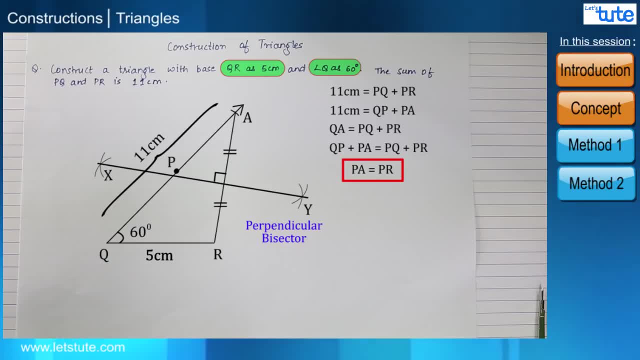 a at a certain point, and this point will be nothing but point B. but why is that so? as per perpendicular bisector theorem, every point on the perpendicular bisector of a segment is equidistant. so point R and point a are equidistant from point P, that is P. a is equal to P. 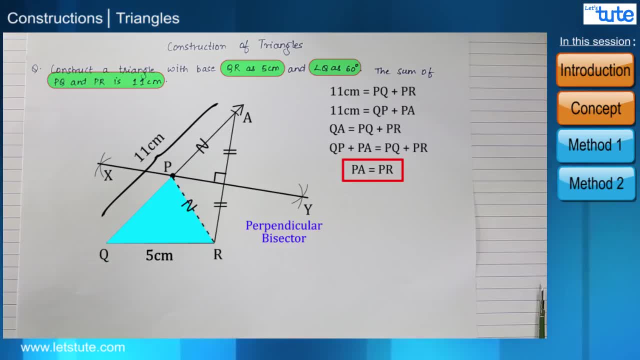 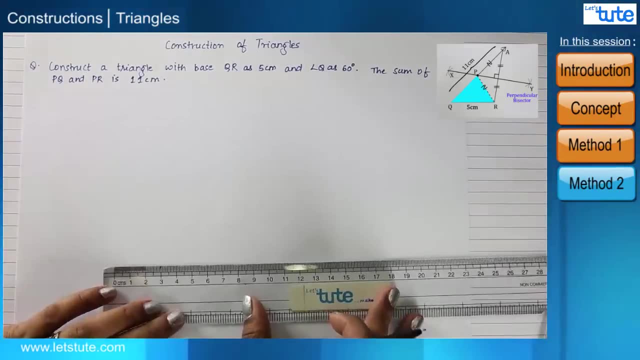 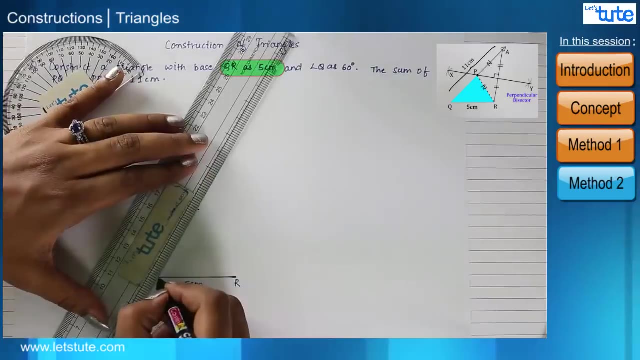 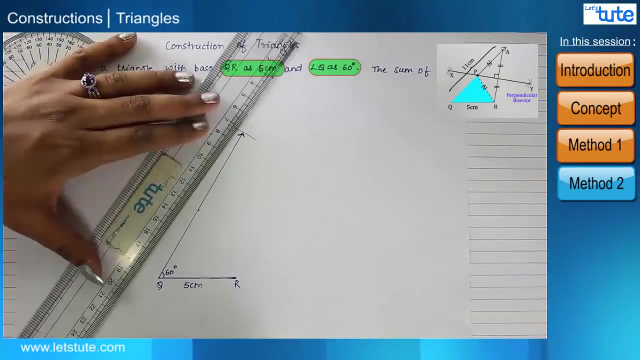 R. so we have gotten our triangle. so let's finally construct our triangle. so the first step will be we'll be drawing base QR as 5 centimeter and angle Q as 60 degrees. now we are going to mark point a and such that Q ay will be equal to P. Q plus P are. well, if we will join a R and 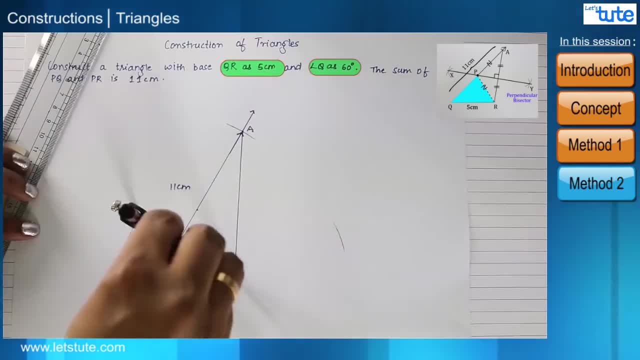 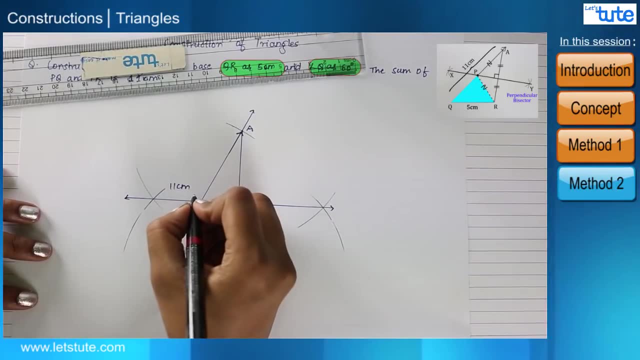 draw perpendicular bisector of the same. now we can see that the perpendicular bisector is cutting segments. you a at this point and this point is nothing but point P. now the last step is: we have to join P R, triangle, P R and point a of the 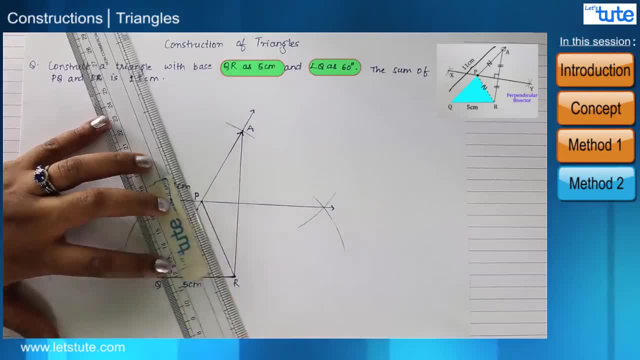 line Q A is even, and trouve a point A of the line Q a of the line Q, and we would have toribulate all論 and we would have toiony and we would have to Opt that we're going to have o Lag here along this string, this line Q A, o Titus seg sob. 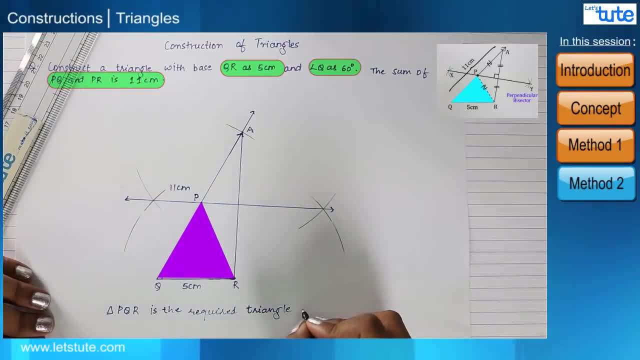 WE DO B? we need to a vin here and B? r even of the line Q a, we need to draw perpendicular. PQR is the required triangle, with base angle as 60 degrees, The base has 5 cm and the length of PQ plus PR is equal to 11 cm. 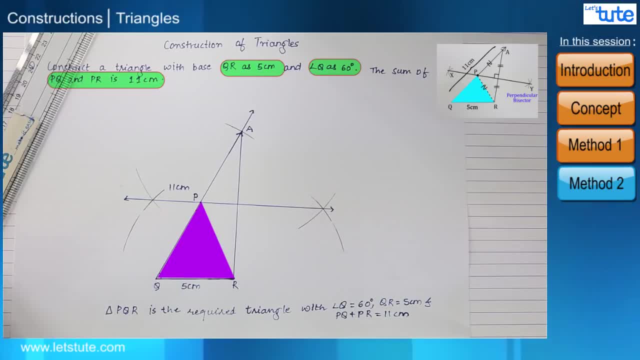 However, there is one more way to draw this triangle with the same given information. Now we know that somehow we need PA is equal to PR. Well, in a triangle, if we need two sides to be equal, then we can get it by drawing two equal angles also. 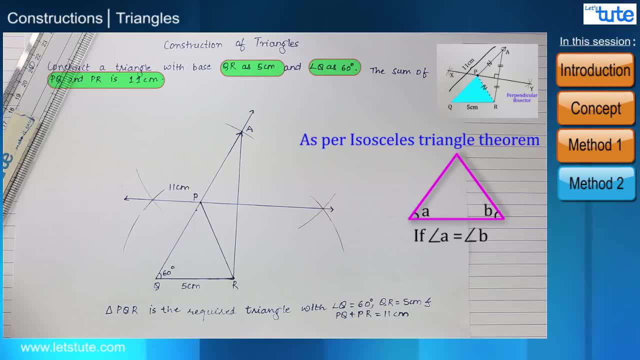 So, as per isosceles triangle theorem, if two angles of a triangle are equal, then the sides opposite to them are also equal. So the first three step will remain the same, that we are going to draw the base QR and make the angle Q. 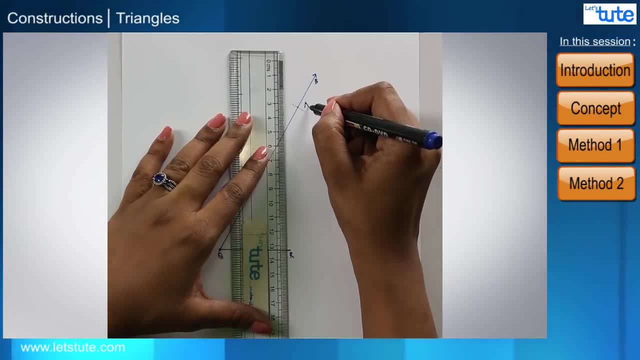 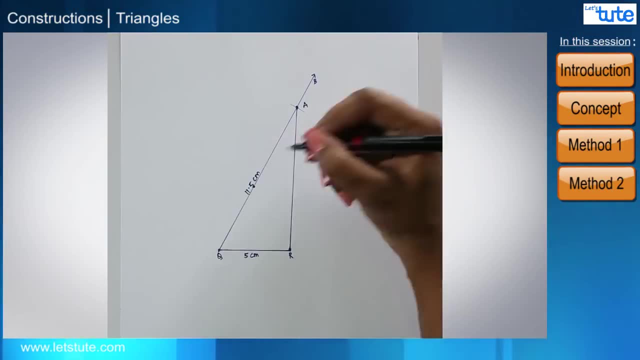 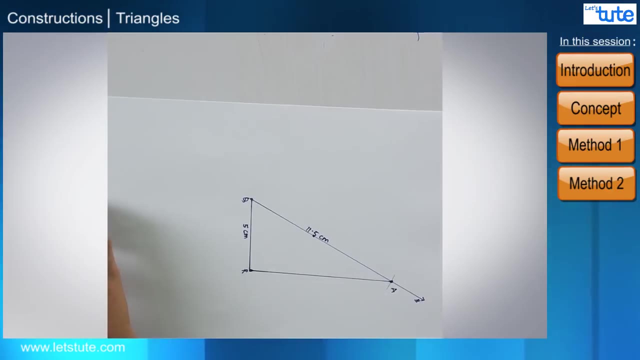 Now we are going to mark point A such that QA will be equal to PQR. So PQR will be equal to PQ plus PR and we will join segment AR. Now we will measure the angle QAR and make an angle of the same measurement from point R. 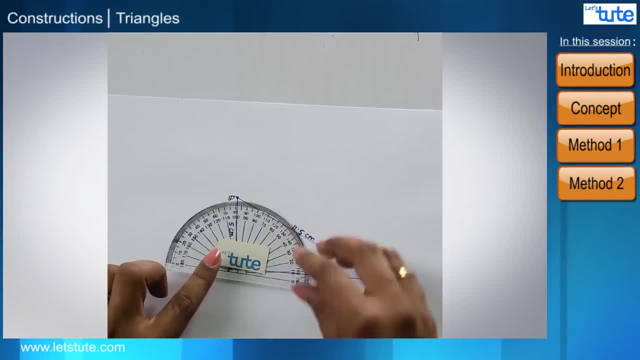 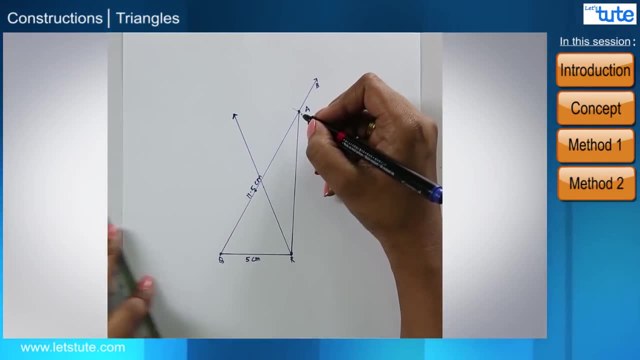 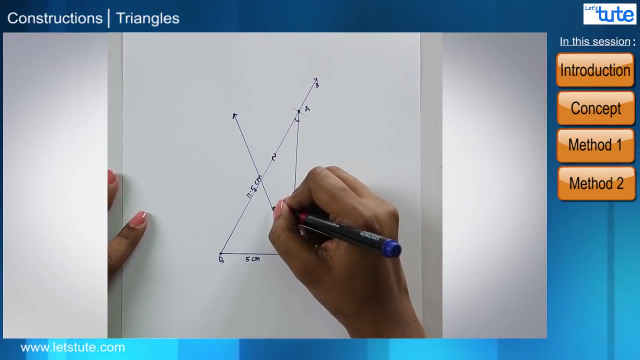 Now here we can see that angle QAR is 25 degrees. So from point R also, we will draw an angle of 25 degrees After extending this ray. we can see that it touches the segment QA. So we can see that it touches the segment QA at a certain point, and this point is nothing but point P and triangle PQR is the required triangle. 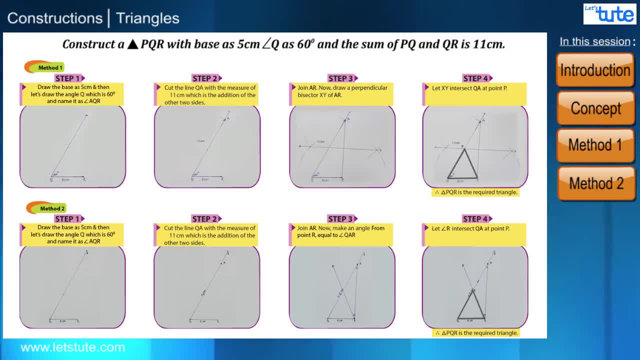 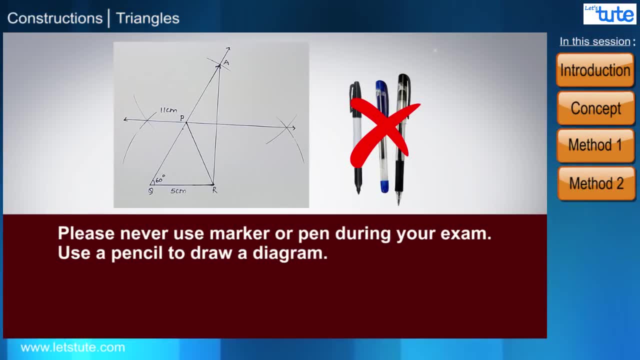 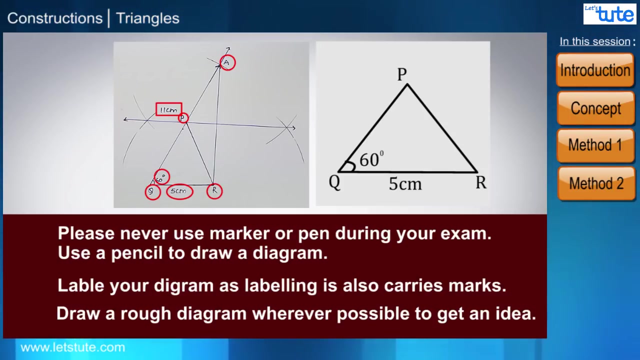 I hope, friends, you have understood this construction and also the mathematical logic behind each of the step. Please, friends, never use a marker or a pen during your exams. Always use a pencil. Always label your diagrams correctly, as the labeling also carries the marks. If possible, draw a rough diagram wherever possible to get a rough idea that how your diagram is going to look like.